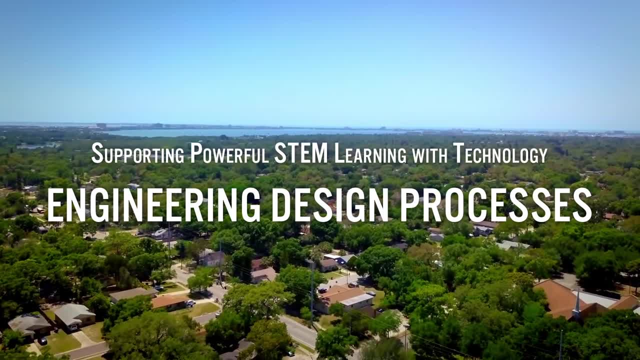 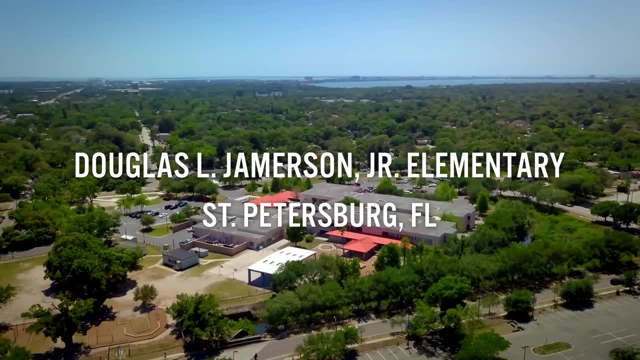 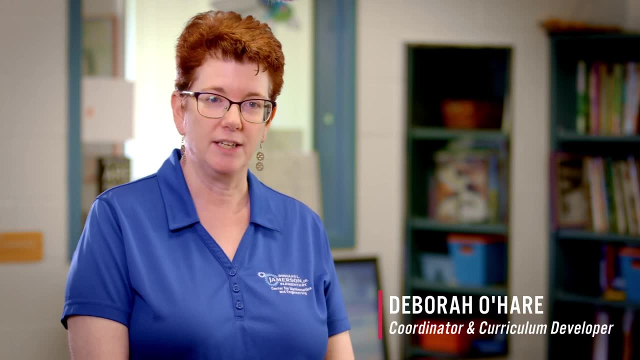 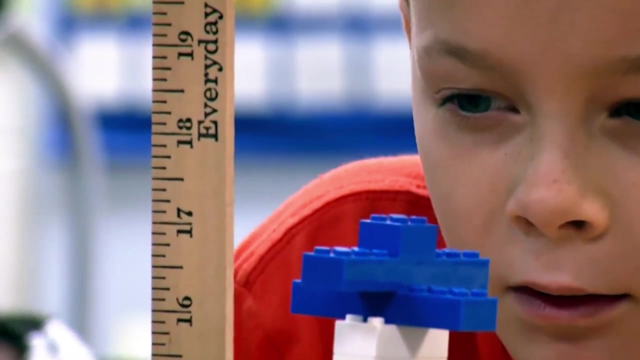 Jamerson Elementary in St Petersburg is the only engineering elementary school in Pinellas County. We focus on a design process, plan, design, check and share. The children learn that starting in kindergarten. We are not here to create little engineers. We are here to teach children how to use the design process to problem-solve and think creatively and how to begin to understand and accept failure. 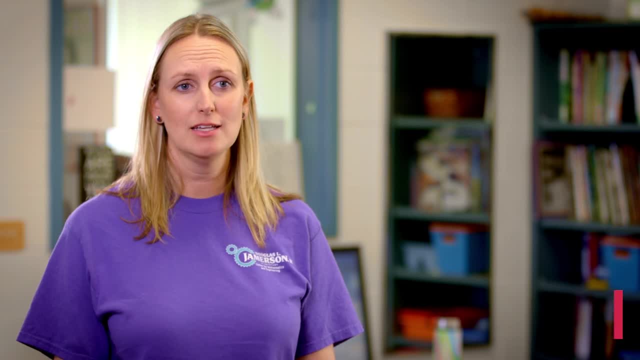 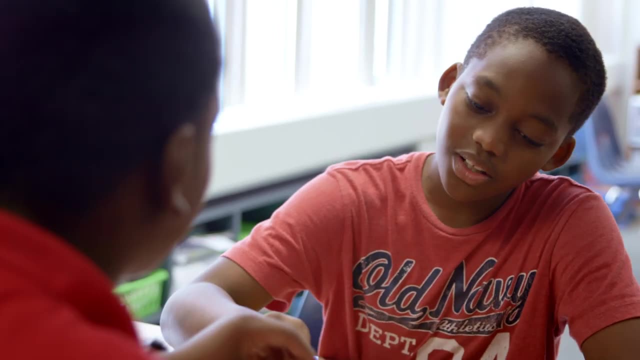 Today the kids were designing insulators and we've done some background labs on insulators and conductors. So the first process in our design challenge is to plan. So the students took all their research and planned together- so drawing it out and talking it through- what they wanted to do. 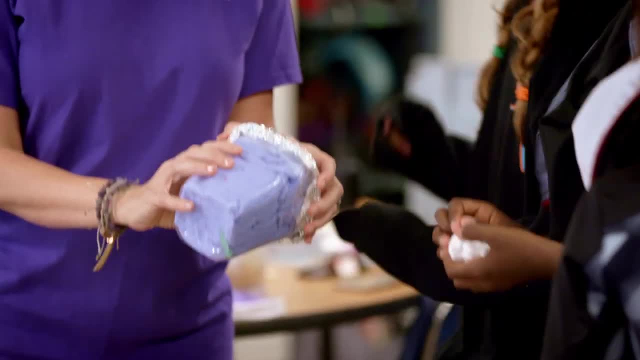 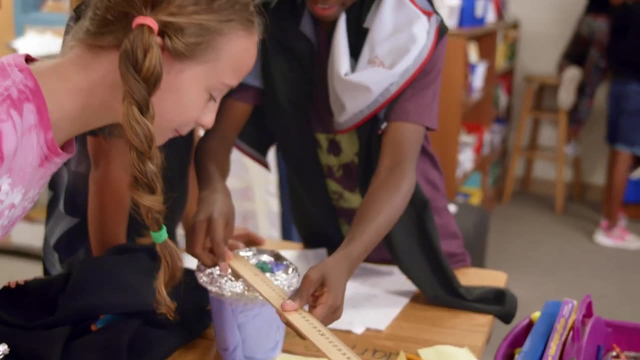 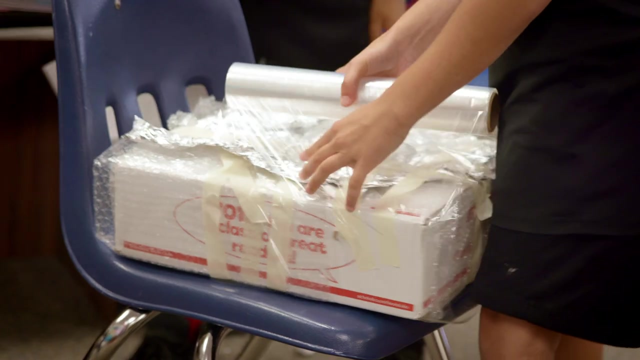 And then they had the two class periods to put everything together and design the actual insulator, What I think we can like make a hole right here. Five, five, six, okay. Working in my team it was actually pretty easy because, like, we can all communicate and we can put in our different ideas and like collaborate with each other. 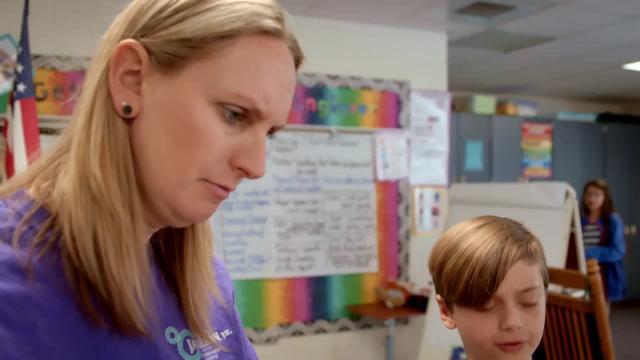 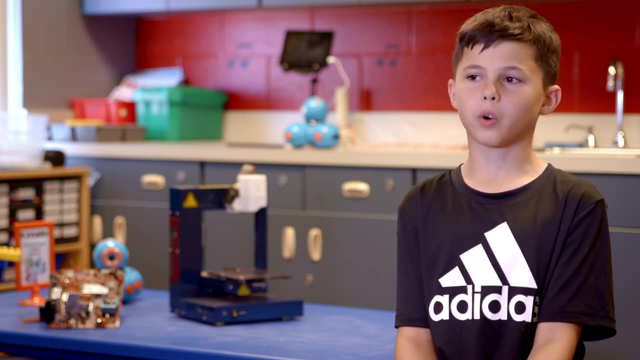 And what was your purpose for the foil on the outside? Um, maybe to, yeah, reflect some of the heat. And we looked back on our third grade skills and we said, when we tested the black and white sheets with thermometers, we figured out that the white had a lower temperature than the black. 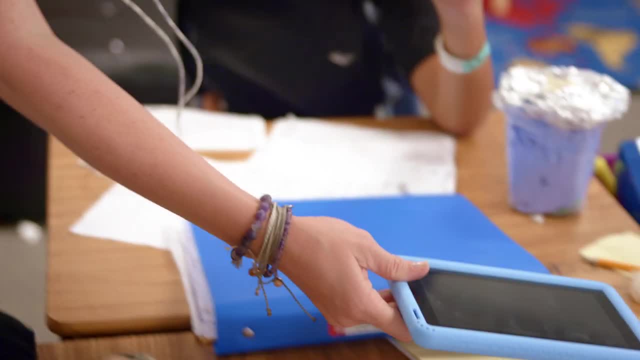 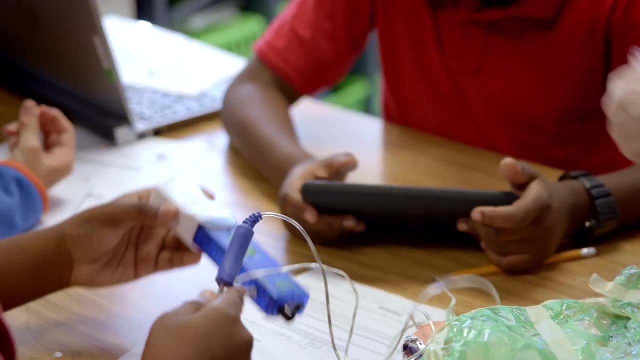 And so we used white blocks. So today was the checking process in our design challenge. They had ice cubes inside trying to keep them from melting. We took the initial temperature before we went out with the probeware. There's your six pieces, put it in, put it in the sun. 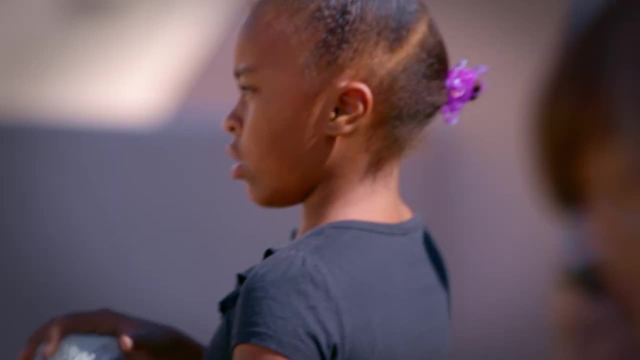 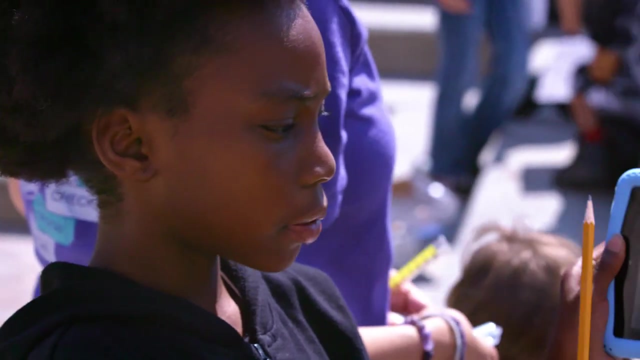 They left it out in the sun for 30 minutes. When the students go on the Kendall, they have to connect it to what they are measuring in units, And so today we were measuring in Celsius, So the probeware was acting as a thermometer to take the temperature of the insulators. 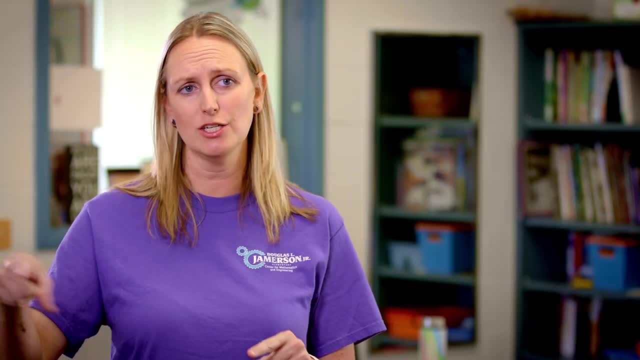 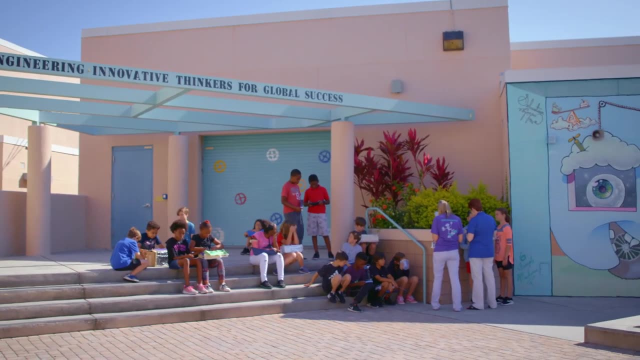 And so then it was reading how much of an increase. It graphed it on a chart, And then they could turn the chart into just a piece of data to write down. Well, with the probe we were able to collect more data easier than with the thermometer.